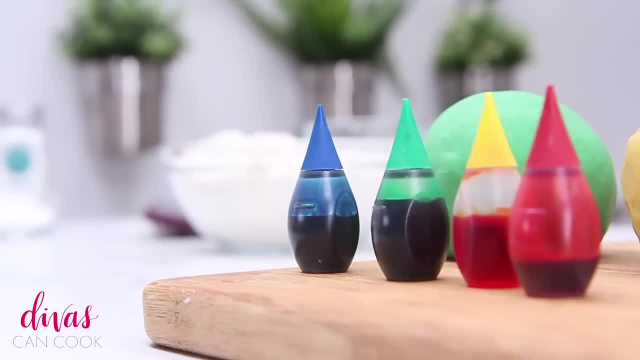 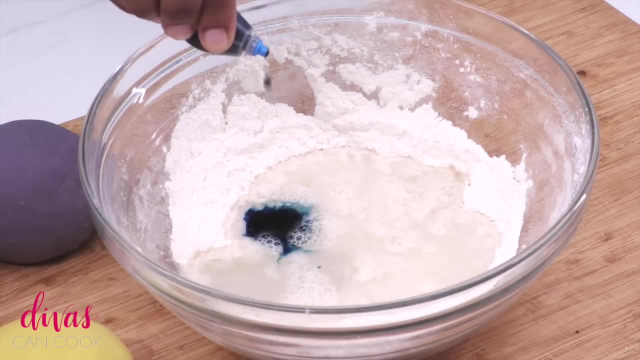 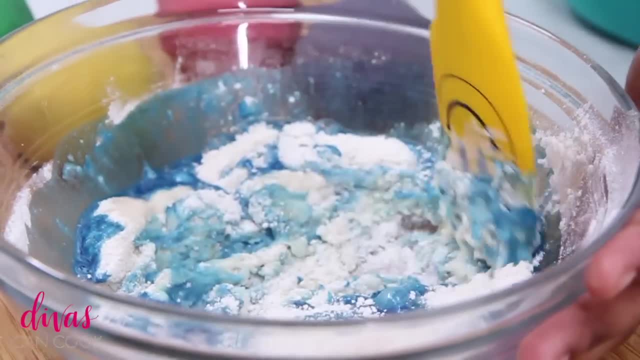 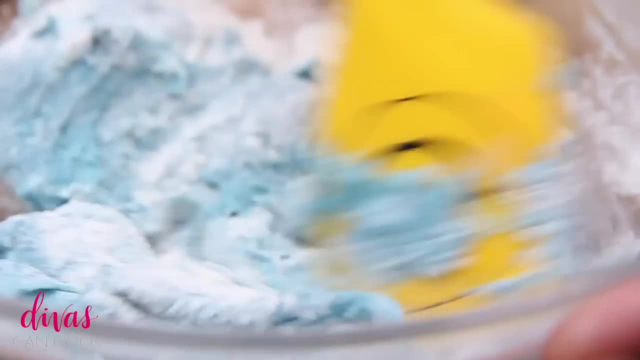 really nice and bold and stuff. Go ahead and stir that up. If you need more flour, add it, but I didn't need any more If it's perfect, just like that. So just use your little spatula to incorporate everything and when the dough is cool enough to touch, go ahead and take it Kind of squish it. 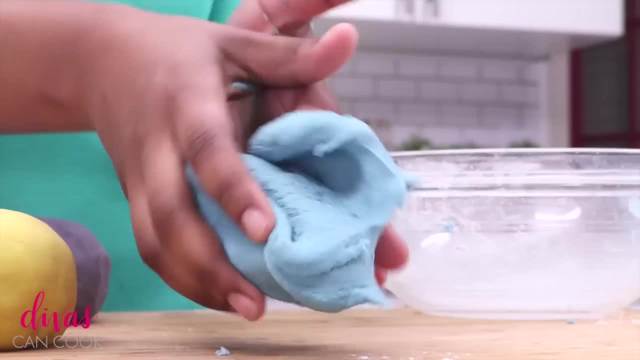 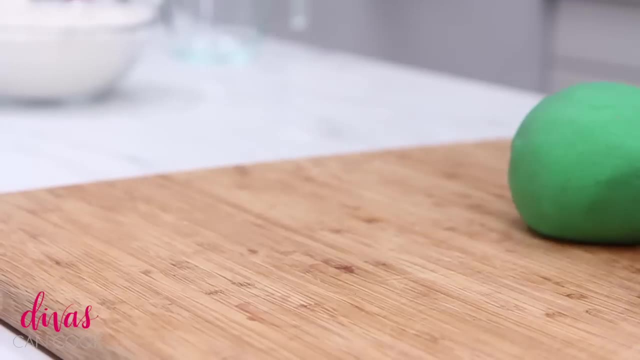 around. This will help really get that flour worked in, and while that dough is warm it'll be kind of sticky, but once it cools down, you're going to have the perfect texture. Oh my god, I can't stop touching this play-doh because it's like the perfect texture ever, and now you are ready to play. 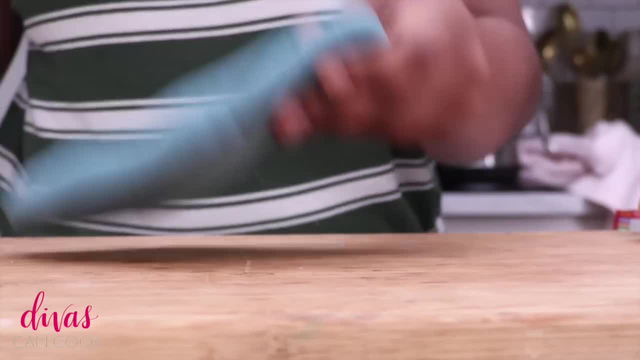 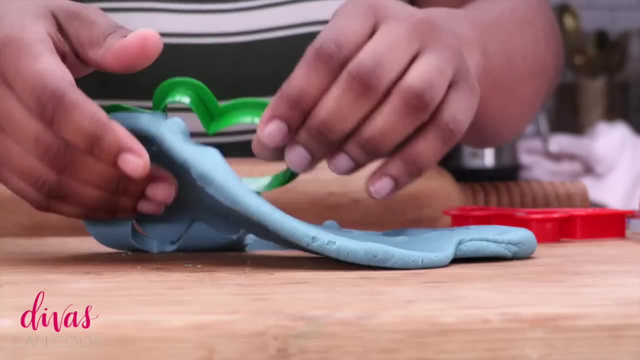 Go ahead and roll it out, It doesn't stick. Oh, it's luscious, luscious, luscious, Perfect for cookie cutters. Yeah, we use a lot of cookie cutters. okay, And it also makes a perfect little snakes because, come on, you got to make. 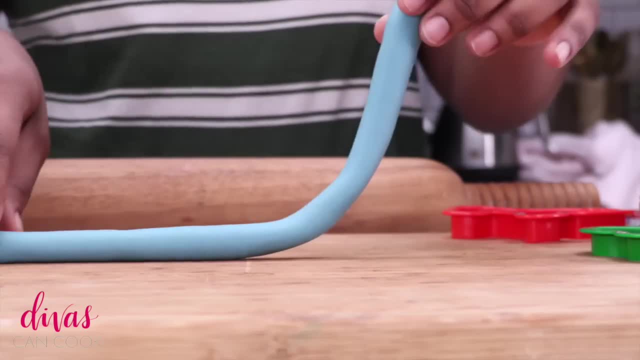 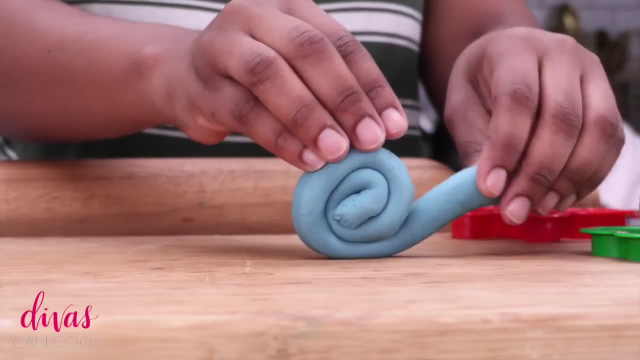 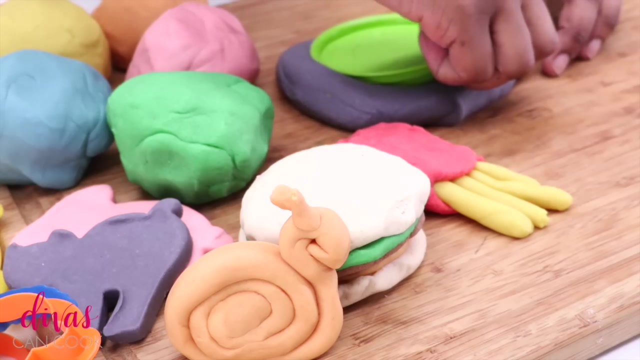 some snakes with play-doh, right? So this play-doh makes a perfect little snakes. It rolls up beautifully, It doesn't crack. Y'all make it because it's so cheap. So go ahead and mix those colors up, Make some food. Play restaurant. I love playing restaurant with my boys and just really. 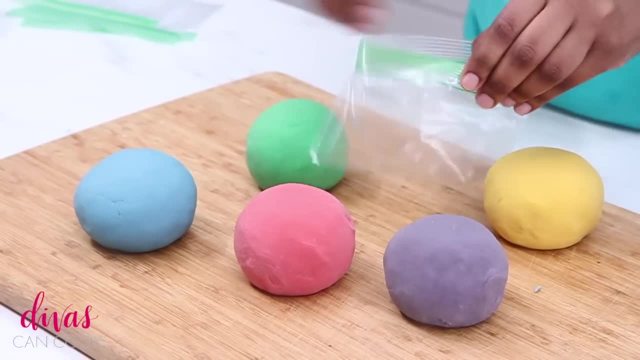 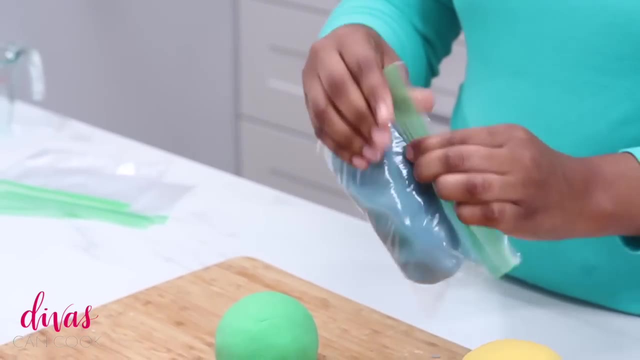 have fun with it. Okay, now to store this play-doh. I like to place it in these little small snack bags, because it makes such small little batches like this. It fits perfectly inside these little snack bags. Go ahead and just seal them on up like that. and also, you guys, if you go to my blog, the 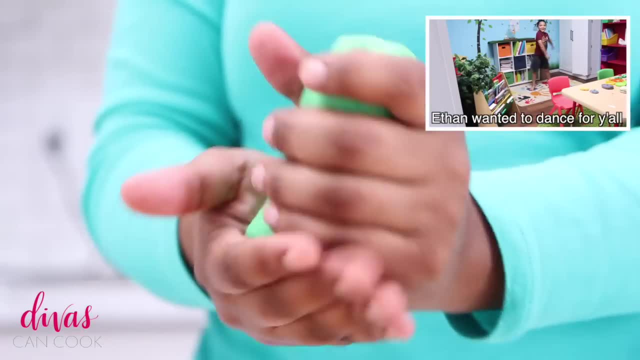 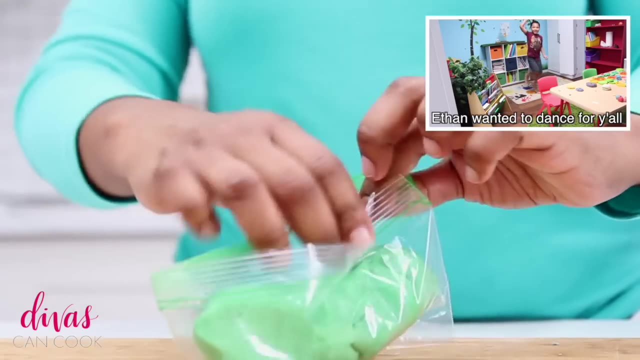 link is below. I have put a whole bunch of fun little resources, things you can do with play-doh, lots of different activities that you can use with play-doh that we, that we who is re-girl that we really really like- Okay, they're nice and sealed up. 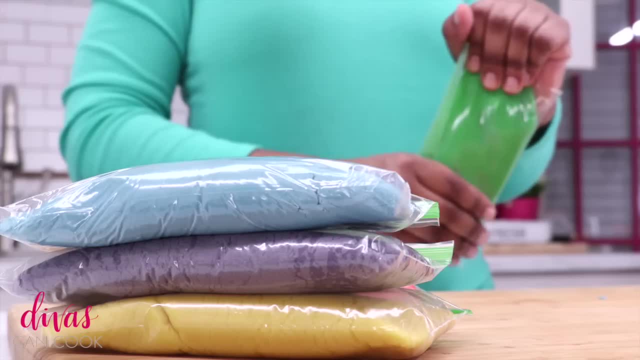 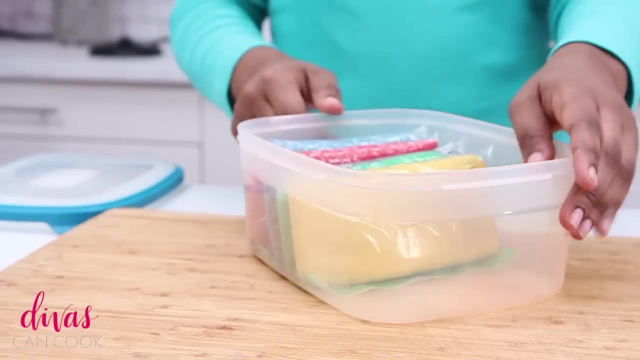 And so cute. Okay, once I have them all sealed up like this, I like to go ahead and place them in a Tupperware container, just to make sure they're double sealed up, because my boys will be closing these bags up. They're not gonna do that. But yeah, this right here, this they can do, All right.